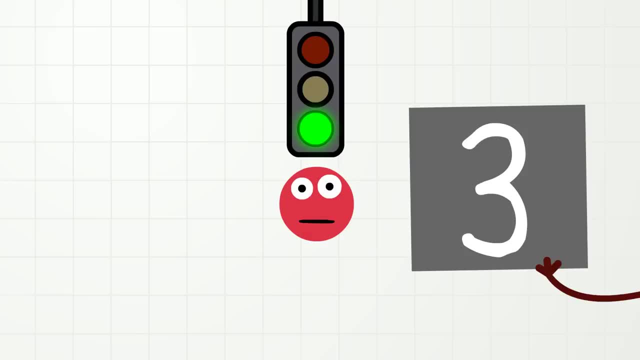 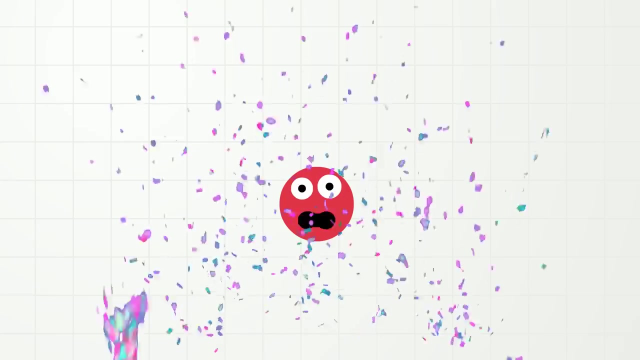 1,, 2,, 3,, 4,, 5,, 6,, 7,, 8,, 9, 10.. Wow, You did such a good job. I think it may be time to celebrate Yay. Ok, that's enough. 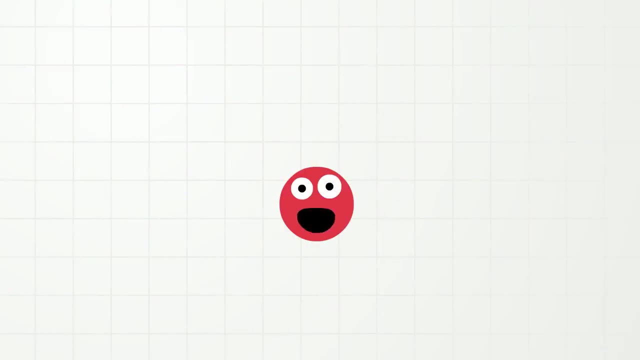 So we can say numbers and we can write numbers, but did you know we can also use numbers to count actual things we see every day? Ha ha, Yes, we can. Let us use an example. What should we use? Hmm, I know How. about spaghetti Spaghetti? Wow, That is a big meatball. Ok, 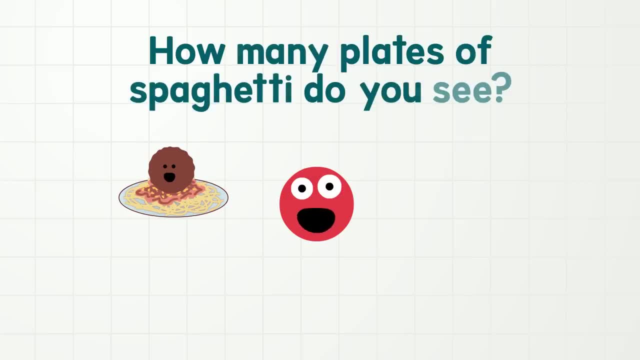 so if I ask you, how many plates of spaghetti do you see? what would you say? That's right. There is one plate of spaghetti. We can say they're one. Woohoo, That's right. There is one plate of spaghetti. We can say they're one. Woohoo, That's right. 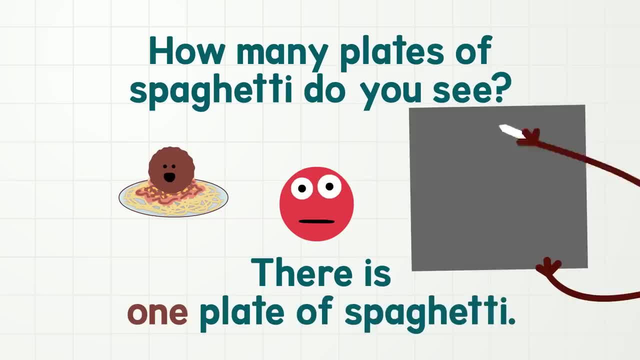 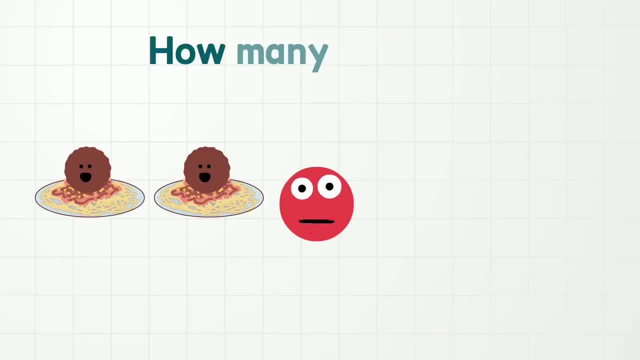 There is one plate of spaghetti. We can say they're one, Woohoo, That's right. There is one plate of spaghetti We can write they're one, Woohoo. And there is actually one plate of spaghetti. See One. Now, how many plates of spaghetti do you see? That's right There. 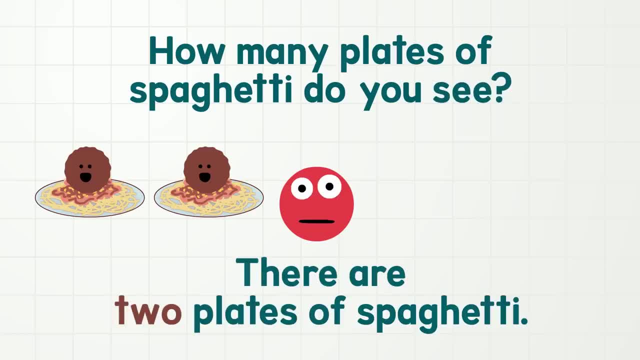 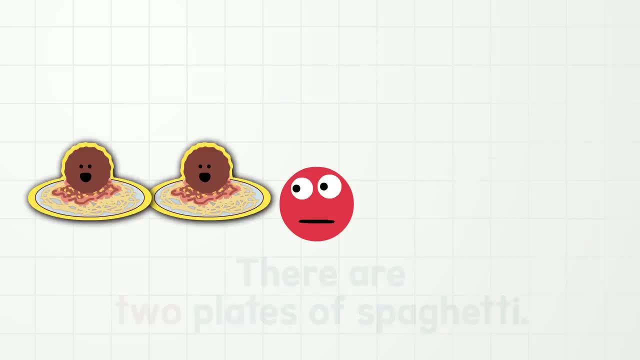 are two plates of spaghetti. We can say two, Two- This is how we write- two, And there are one, two plates of spaghetti. So now let's count to 10 again together, while watching the plates of spaghetti. Okay, ready. 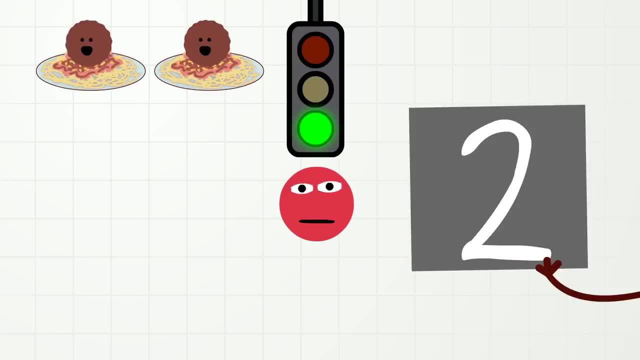 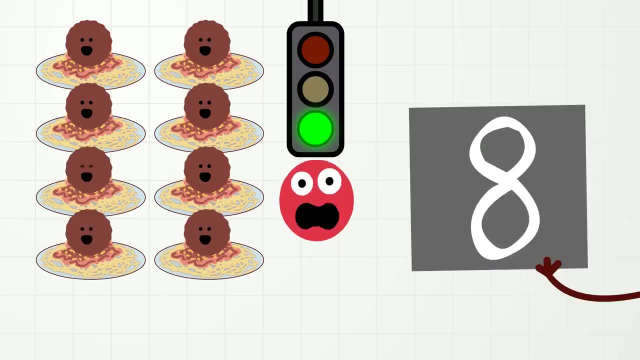 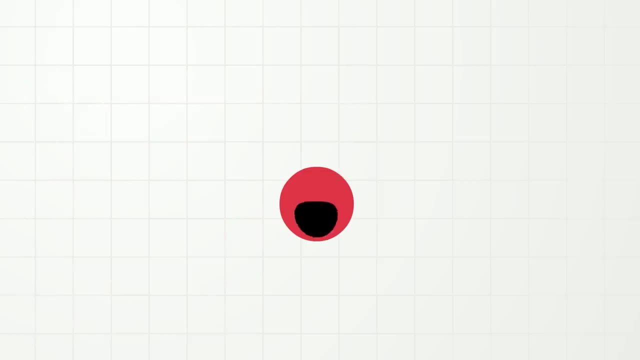 Go: 1,, 2,, 3,, 4,, 5,, 6,, 7,, 8,, 9, 10.. Oh great, I think you really like spaghetti. Now let's count something else. 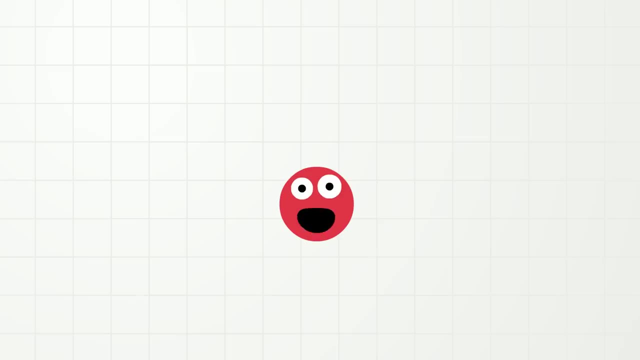 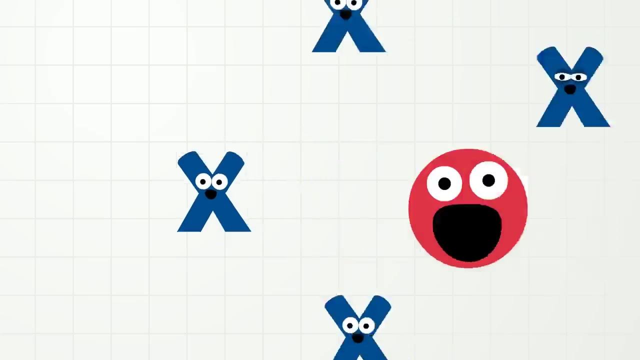 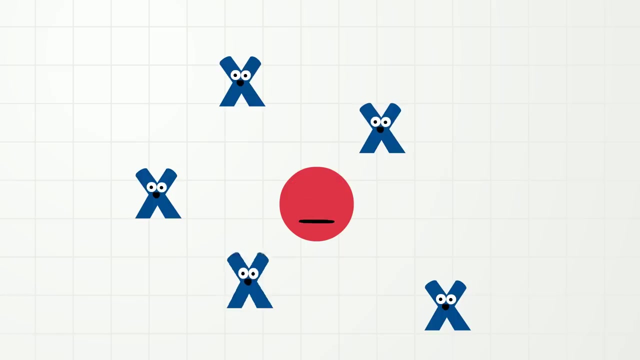 Hmm, how about the letter X? I said letter X, Say hi to the letter X. How many letter Xs do you see There are, let's count- 1, 2,, 3,, 4, 5.. 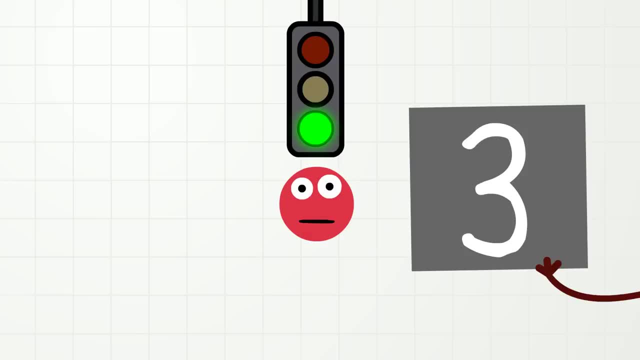 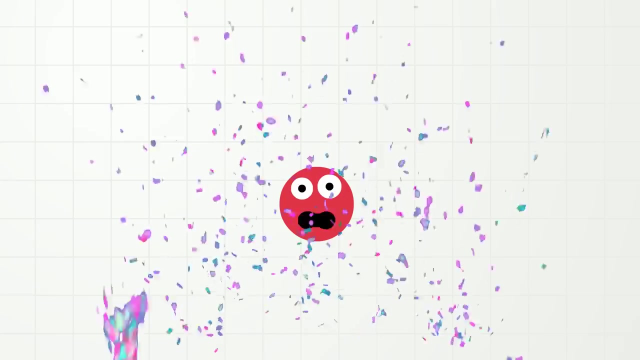 1,, 2,, 3,, 4,, 5,, 6,, 7,, 8,, 9, 10.. Wow, You did such a good job. I think it may be time to celebrate Yay. Ok, that's enough. 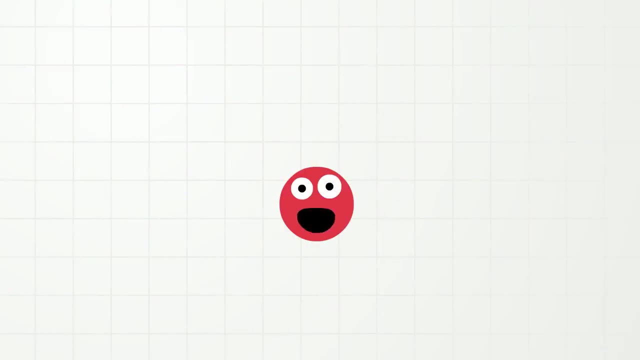 So we can say numbers and we can write numbers, but did you know we can also use numbers to count actual things we see every day? Ha ha, Yes, we can. Let us use an example. What should we use? Hmm, I know How. about spaghetti Spaghetti? Wow, That is a big meatball. Ok, 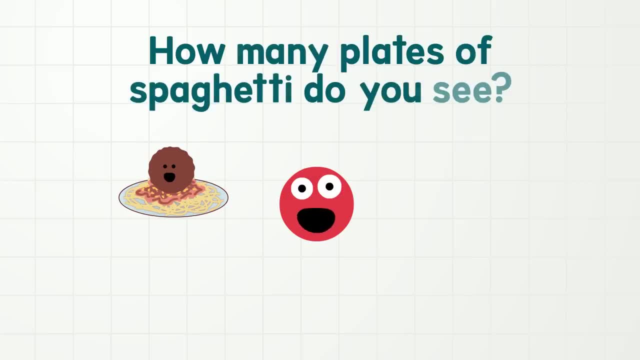 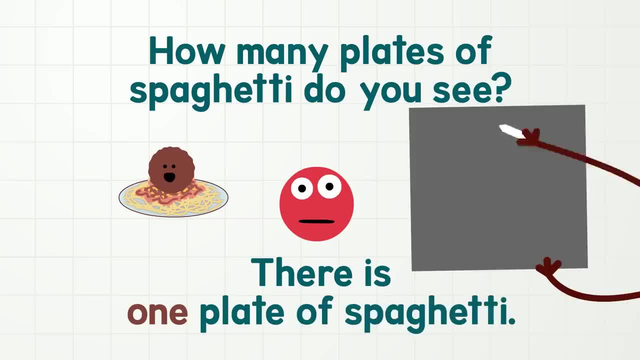 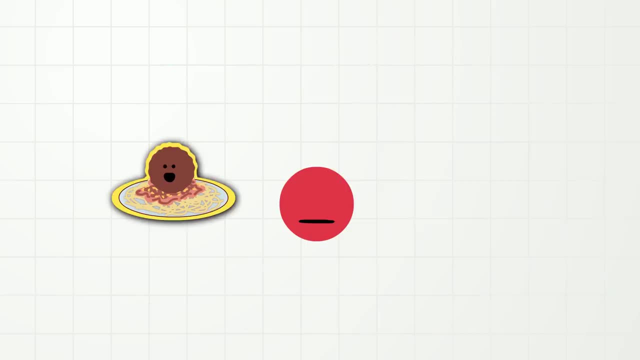 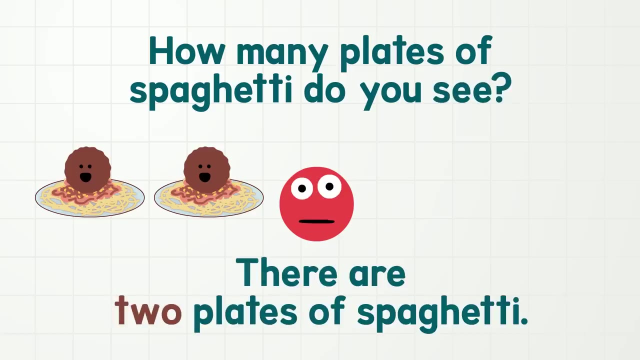 one plate of spaghetti. See One. Now, how many plates of spaghetti do you see? That's right. There are two plates of spaghetti. We can say two, Two, This is how we write- two, And there are one, two plates of spaghetti. So now let's count to ten, again together while. 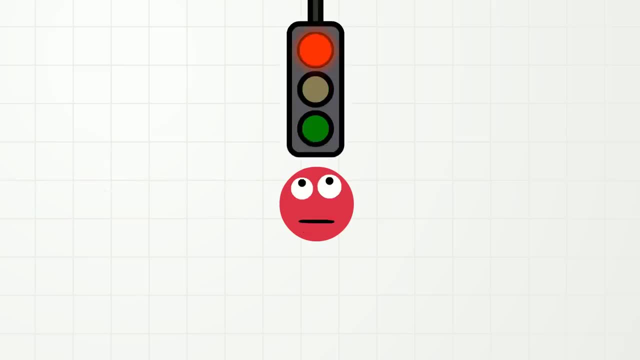 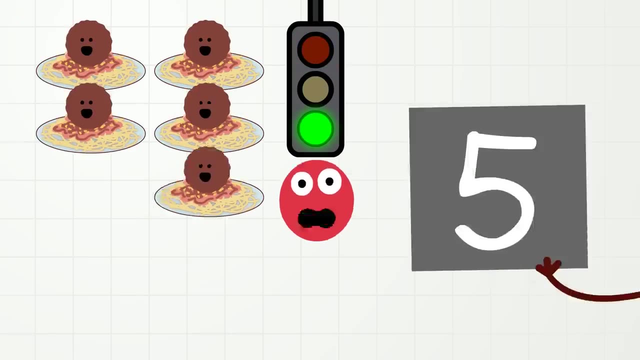 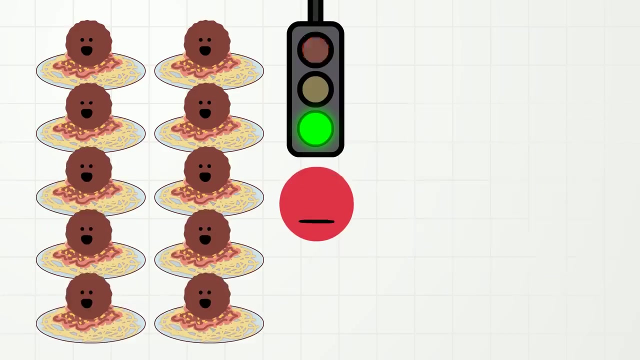 watching the plates of spaghetti. Okay, ready, Go. 1, 2,, 3,, 4,, 5,, 6,, 7,, 8,, 9,, 10.. Oh great, I think you really like spaghetti. 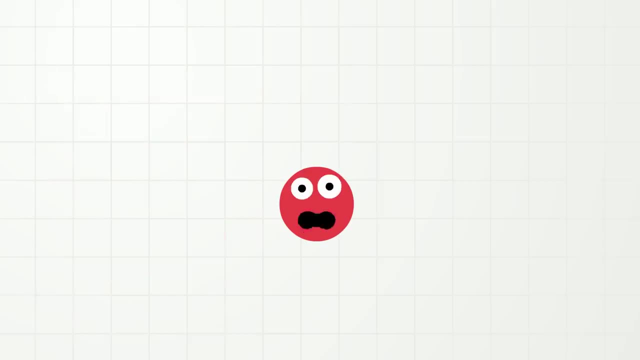 Now let's count something else. Hmm, how about the letter X? I said letter X, Say hi to the letter X. How many letter Xs do you see There are? Let's count: 1,, 2,, 3,, 4,, 5.. 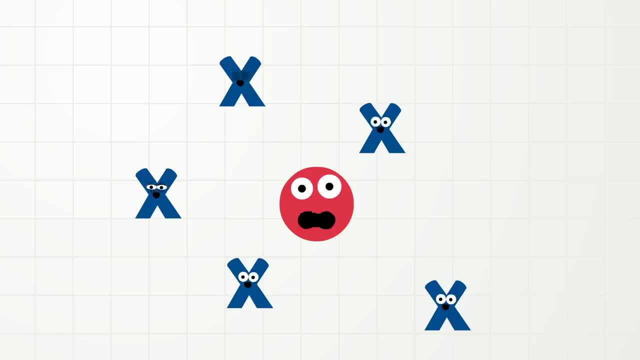 There are five letter Xs. We can say five, Five And we can write five, And we know from counting them. there are actually five letter Xs, See 1, 2,, 3,, 4, 5.. 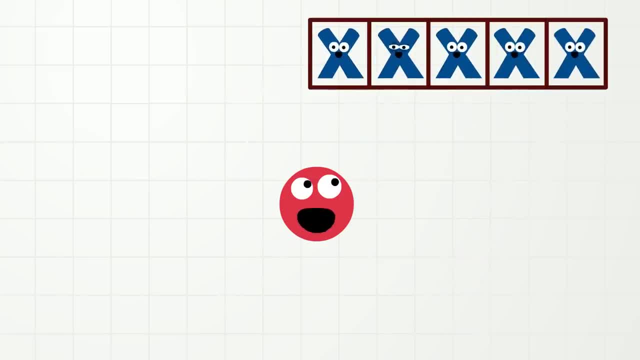 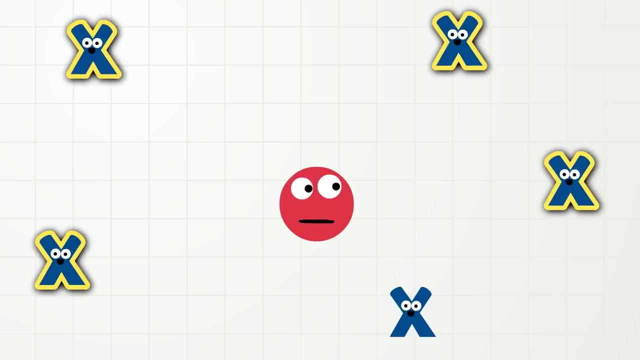 So, even if the Xs go all the way over there, there are still five: 1, 2,, 3,, 4, 5.. And even if they are spread out, there are still five: 1,, 2,, 3,, 4, 5.. 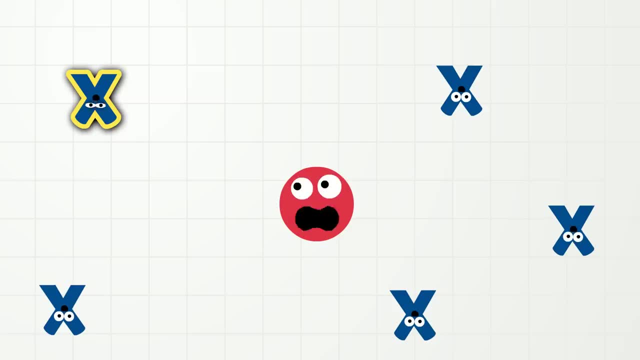 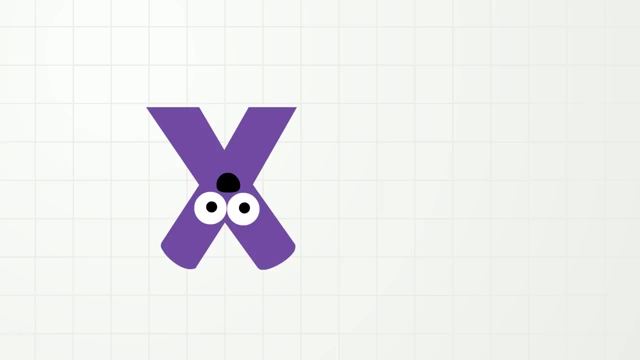 Even if they are upside down, there are still five: 1,, 2,, 3,, 4, 5.. Even if they are upside down, purple, with green polka dots and all with mustaches, there are still five. 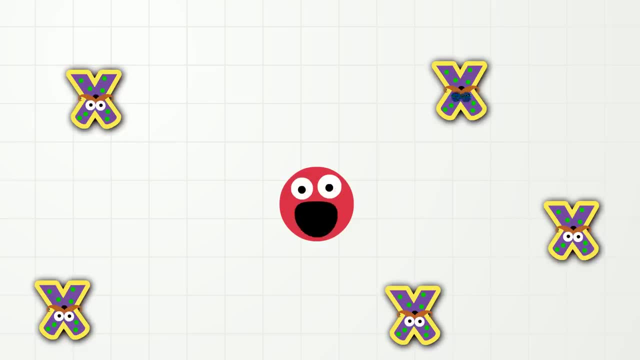 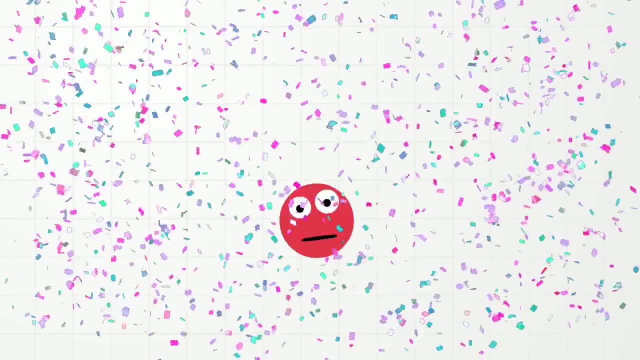 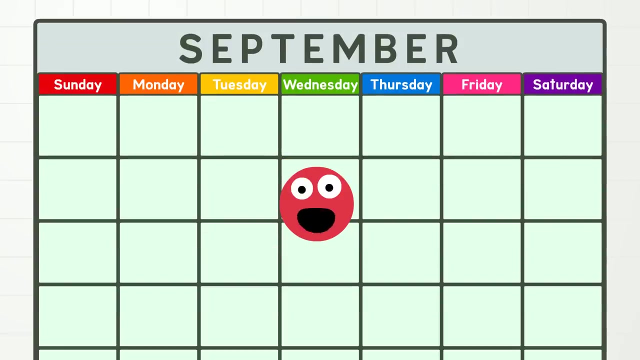 One, two, three, four, five. Ho ho, Good job counting. I think it may be time to celebrate, Yay. Okay, that's enough. Now let's find something else to count Here. do you know what this is? 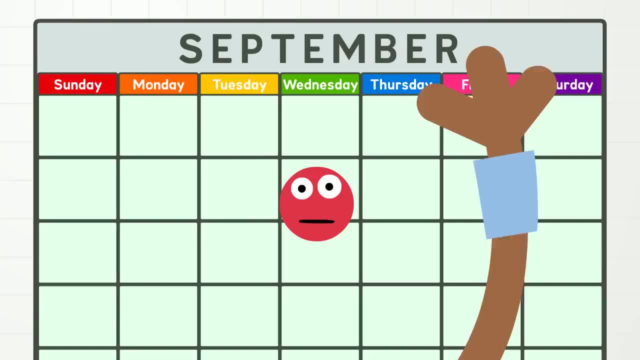 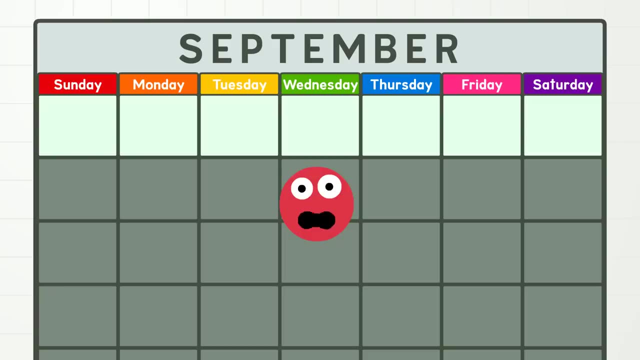 Is it a plate of spaghetti? No, it is a calendar. Uh, that's what I said: A calendar. No, you did not. Anyway, a calendar shows you all the days and all the weeks of a month. Let us look at just one week and try and count the days. 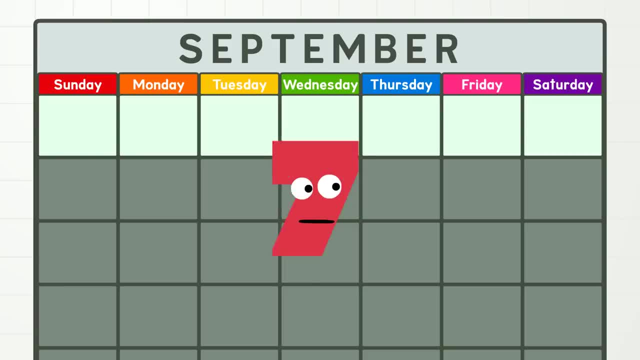 Do you know how many days there are in one week? Seven. Let us count how many days there are in a week together, Ready Go: One, two, three, four, five, six, seven, eight, nine, 10,, 11,, 12,, 13,, 14,, 15,, 16,, 17,, 18,, 19,, 20,. 21,, 22,, 23,, 24,, 25,, 26,, 27,, 28,, 29,, 30,, 31,, 32,, 33,, 34,, 35,, 34,, 35,, 35,, 36,, 37,, 38,, 39,, 40,, 41,, 42,, 41,, 44, And. 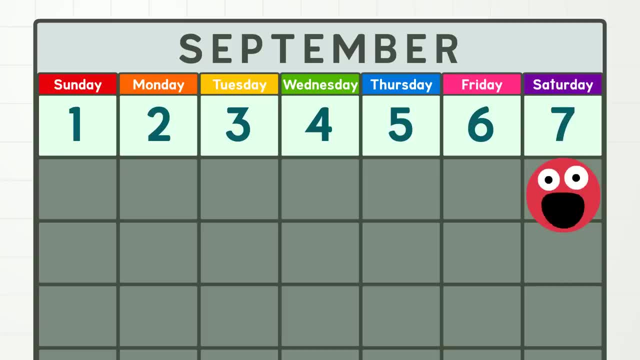 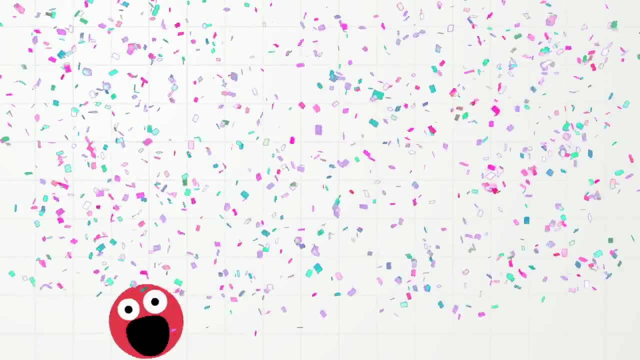 a second mark: One, two, three, four, five, six, seven. wow, You did so great that I think it may be time to celebrate Yay. Okay, that's enough. Oh, don't forget to subscribe to our channel for more laughing and learning from Scratch. 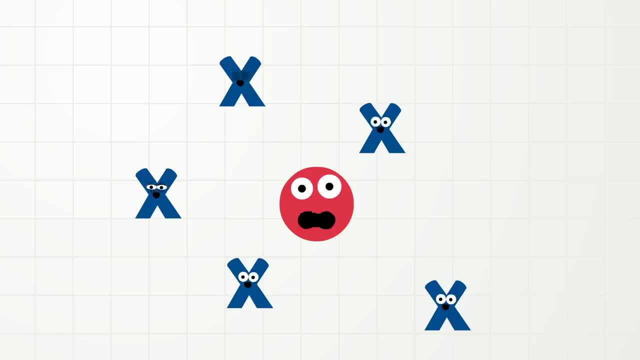 There are five letter Xs. We can say five, Five And we can write five And we know from counting them. there are actually five letter Xs, See 1,, 2,, 3,, 4. 5. 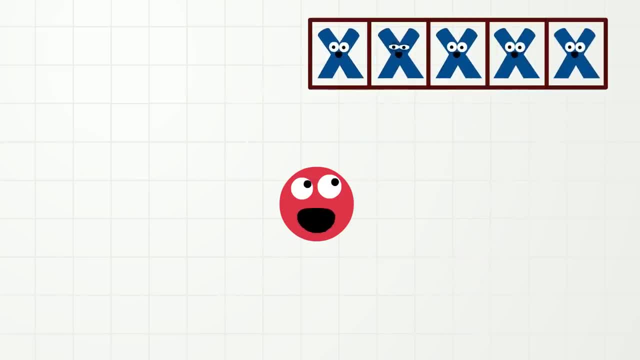 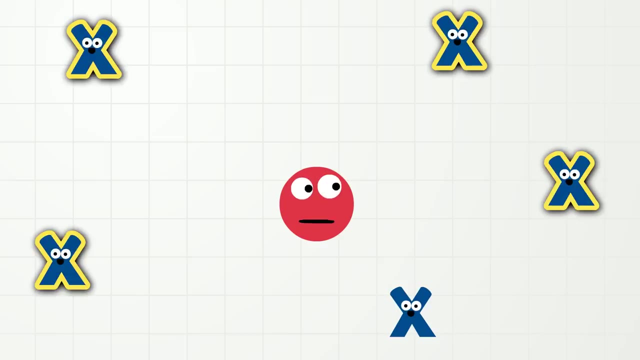 So, even if the Xs go all the way over there, there are still five: 1, 2,, 3,, 4, 5.. And even if they are spread out, there are still five: 1,, 2,, 3,, 4, 5.. 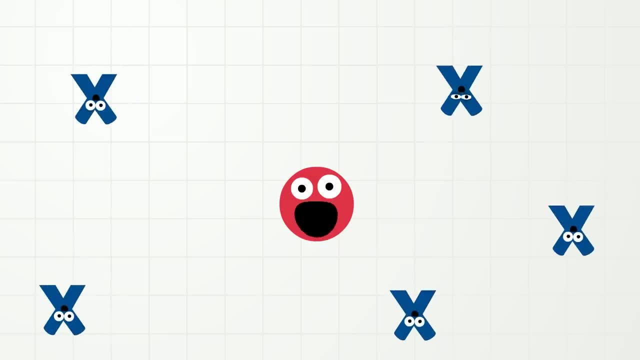 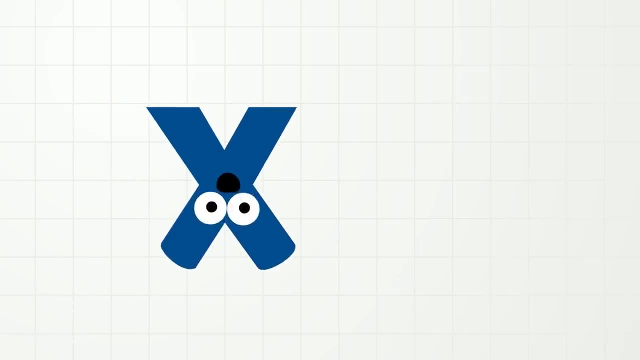 Even if they are upside down, there are still five: 1,, 2,, 3,, 4, 5.. Even if they are upside down, there are still five. Upside down. purple with green polka dots and all with mustaches: there are still five. 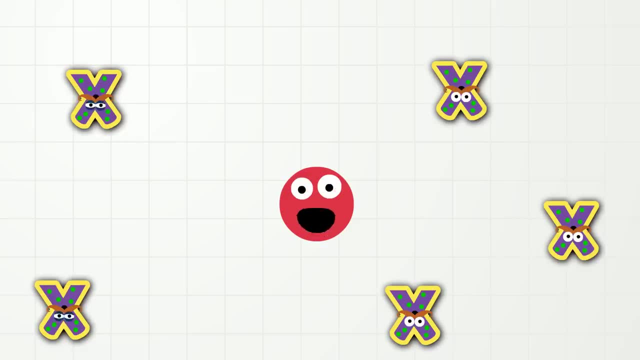 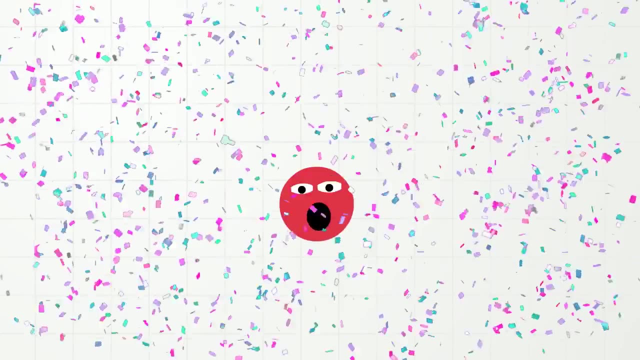 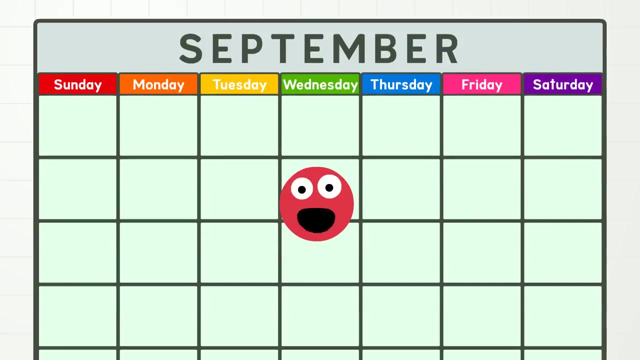 One, two, three, four, five. Ho ho, good job counting. I think it may be time to celebrate, Yay. Okay, that's enough. Now let's find something else to count Here. do you know what this is? 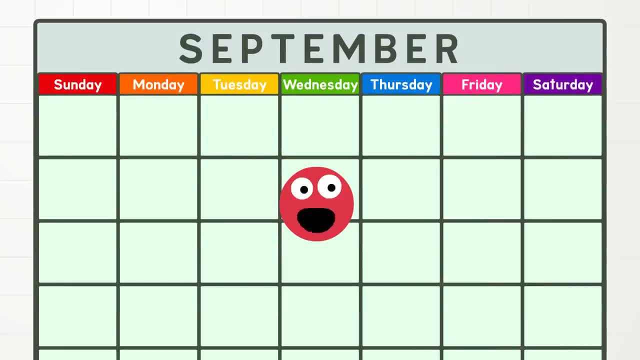 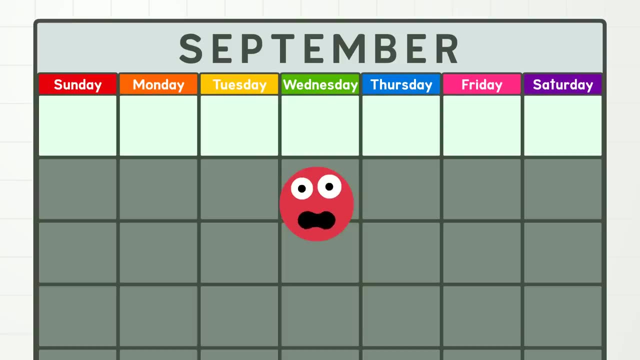 Is it a plate of spaghetti? No, it is a calendar. Uh, that's what I said: a calendar. No, you did not. Anyway, a calendar shows you all the days and all the weeks of a month. Let us look at just one week and try and count the days. 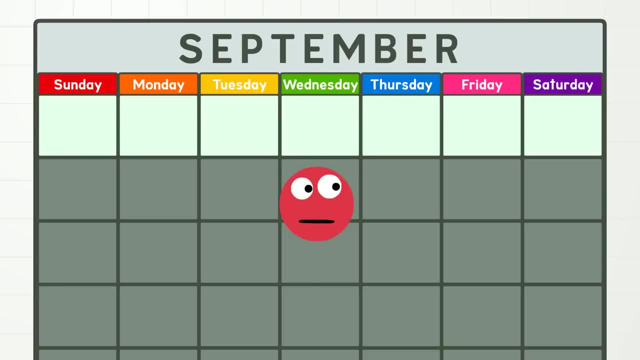 Do you know how many days there are in one week? Seven. Let us count how many days there are in a week together: Ready Go, One, two, three, Four, five, six, seven. Wow, you did so great that I think it may be time to celebrate. 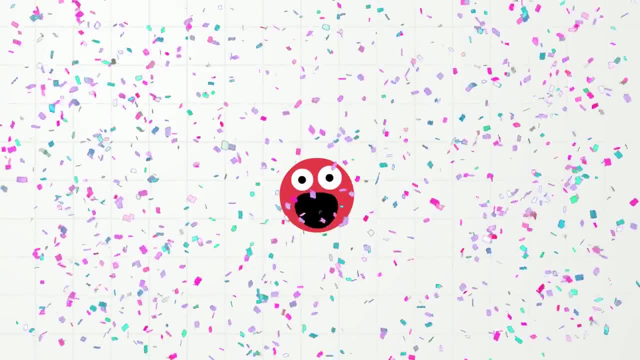 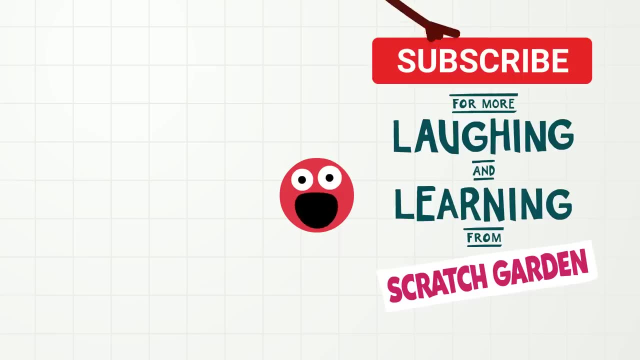 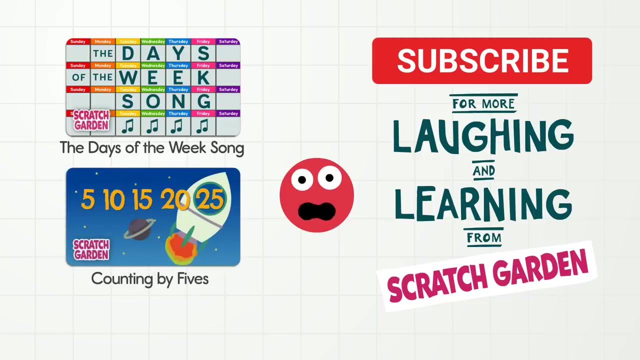 Yay, Okay, that's enough. Oh, don't forget to subscribe to our channel for more laughing and learning from Scratch Garden. And did you know that we have other videos on days of the week and on counting, And we have, like so many counting videos? 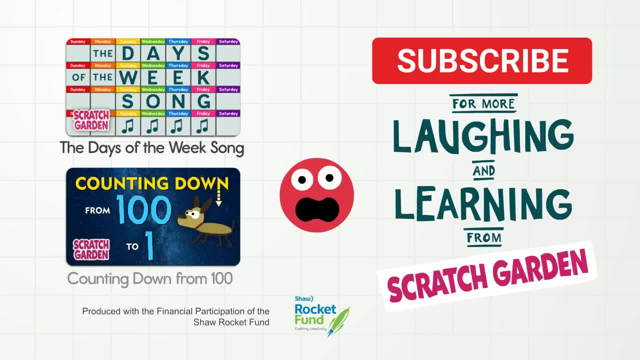 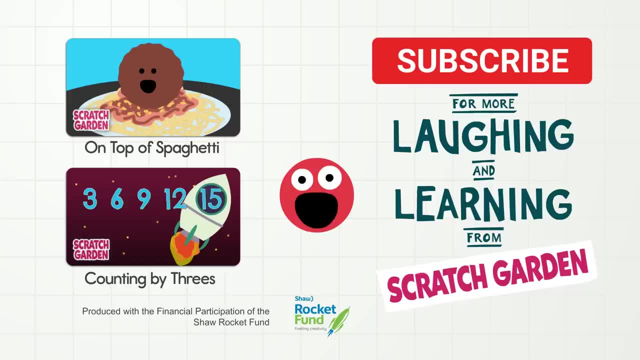 You may even have to help me count how many We have. so many counting videos we have, And we also have videos about spaghetti. No, I am serious. Okay, bye for now. Bye for now.